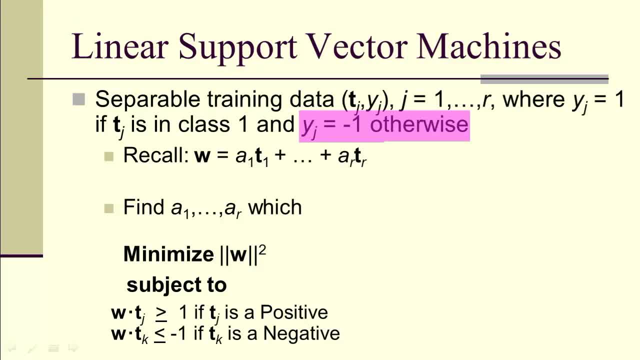 Notice that I've changed to y sub j equals negative 1 instead of y sub j equals 0, because it's going to allow us to rewrite our conditions as simply y sub j times the quantity w dot t sub j greater or equal to 1 for both the positives and the negatives. 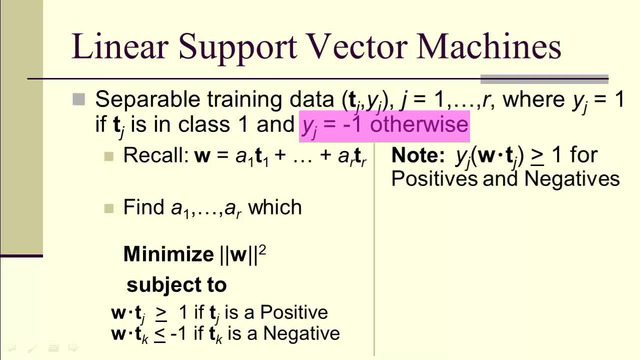 So in other words, both those inequalities are implied by this single inequality. So we're going to do that As long as we have y sub j equals 1 for class 1 and negative 1 for not in class 1.. 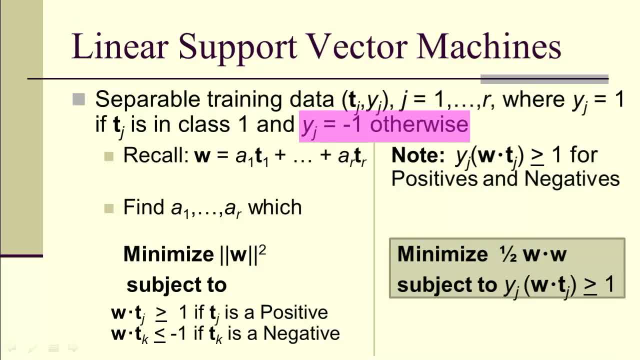 So now we've got this nice little problem. We want to minimize one half w dot w The one half there is for mathematical convenience. In particular, take a derivative of something squared: a 2 pops out. the 2 and a half will cancel. 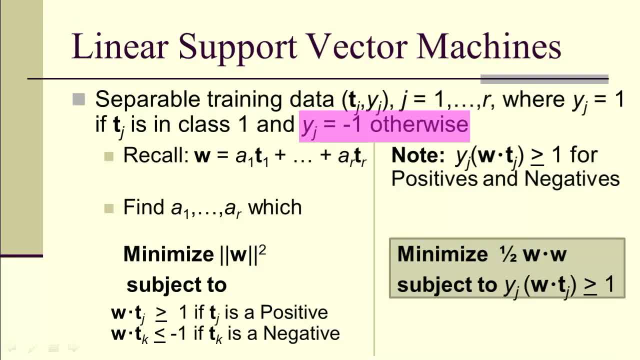 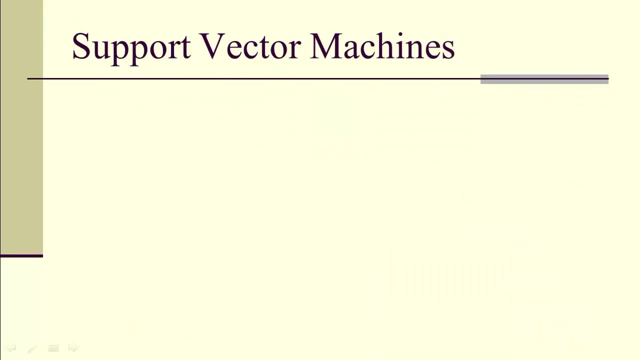 We won't have to worry about the constant factor there- And subject to This boundary condition or this constraint for all the different features. So let's just remind ourselves of our notation. So a support vector machine. the goal is if it's separable, but not linearly separable. 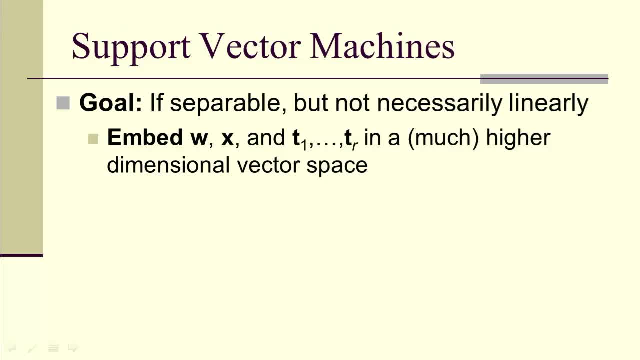 maybe we can project upwards, Maybe we can project upwards, Maybe we can project upwards Into a much higher dimensional vector space. So we can take our feature vectors and our x's and our parameter vector w And we can go up into a much larger vector space. 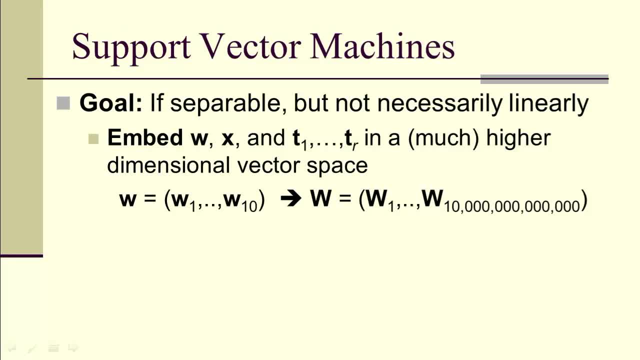 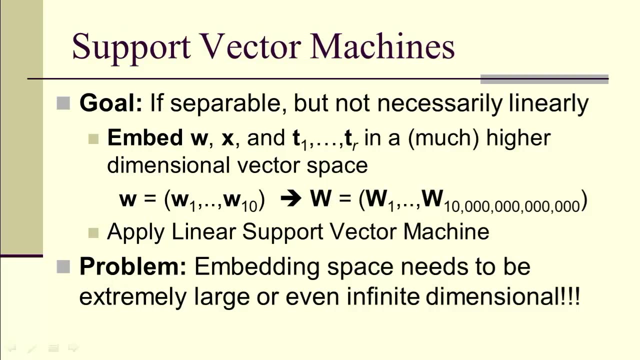 Maybe from a 10 dimensional vector space to a 10 trillion dimensional vector space And then apply the linear support vector machine in the 10 trillion dimensional vector space. Now what we're going to see is that the embedding space to actually pull this off tends to be very, very large or even infinite dimensional. 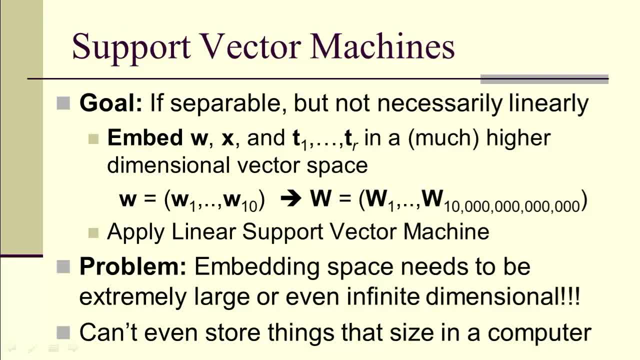 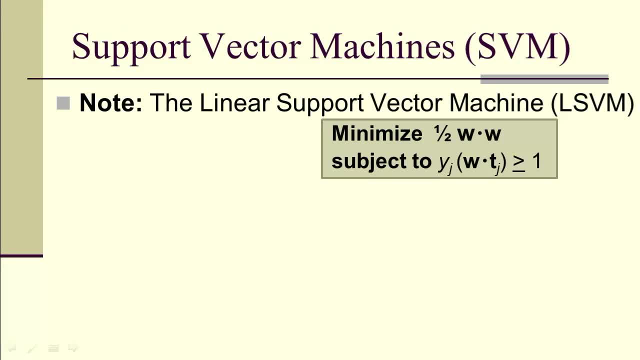 Now you can't store things that size in a computer, So explicitly doing this embedding is pretty much impossible. But again there's a trick. So linear support vector machine: minimize one half w dot w Subject to, Subject to that boundary condition that you see. 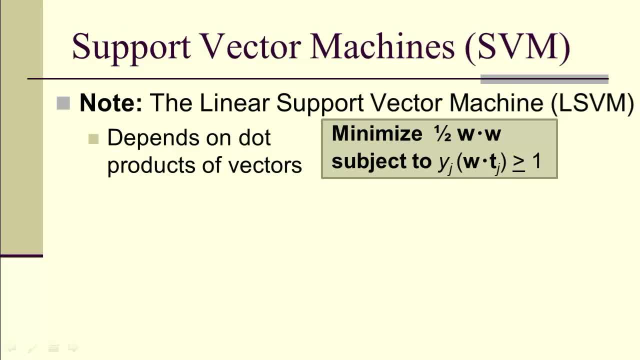 That constraint Notice. this entire problem depends only on the dot product of vectors. Every vector that occurs inside the problem is actually also inside a dot product. There's no vectors kind of hanging out by themselves. So if we've got w equals k equals 1 to r of a sub k, t sub k, the linear combination of the t sub k's, it's the same thing. 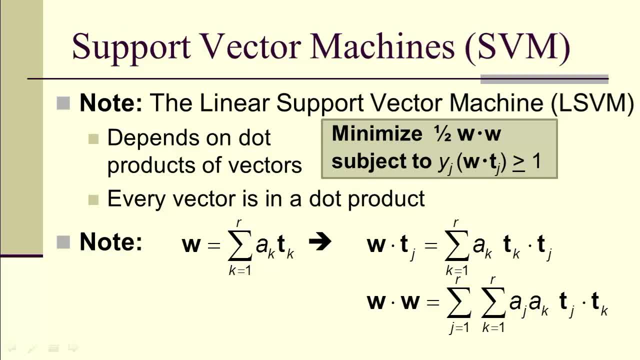 So the only time we see a vector is when it's inside of an inner product And w, dot w is a product of the linear or the scalar coefficients a, sub j, a sub k times a dot product. So we can minimize over these scalars. 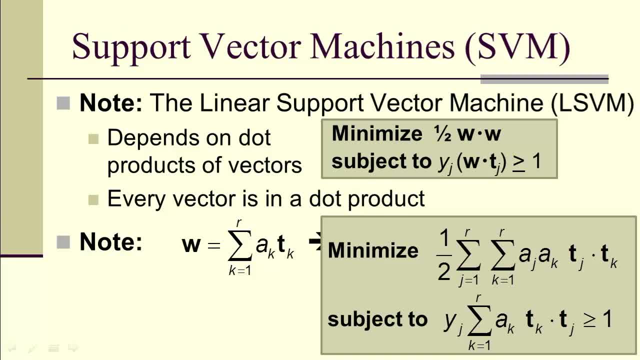 a sub j, for j equals 1.. So now we have u: 3 through j equals the number of separators. We can step it up to r And we can rewrite our constraint in terms of the scalars, And since now we have a problem that's over scalars. 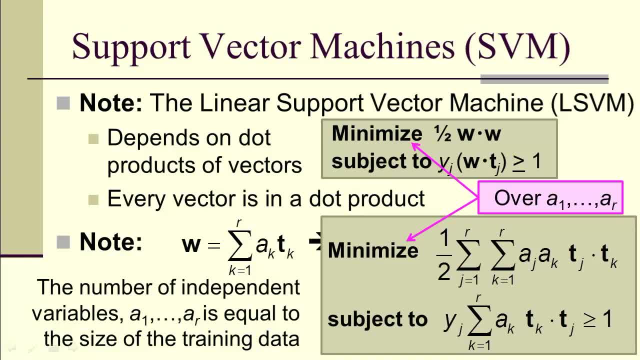 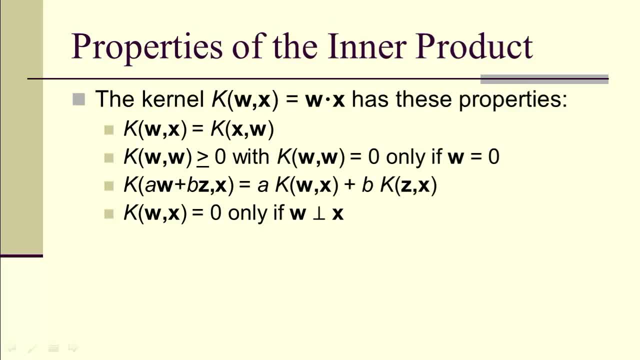 then, essentially, the number of independent variables, which are the scalars, is equal to the size of the training data. Now, what properties does an inner product have? Well, you, something like this, you have to have symmetric, the inner product of W, with 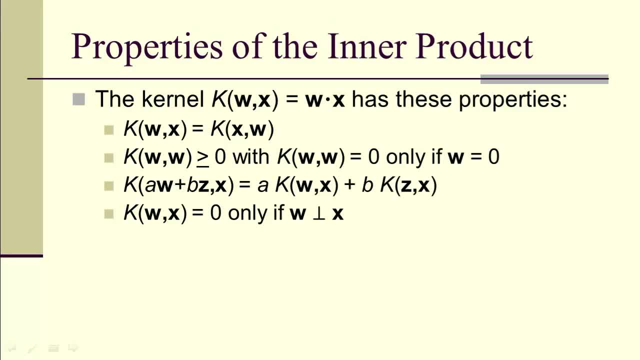 itself has to be non-negative. it can be 0 only if W- 0, the inner product is linear. in the first argument and they'll also explain: you know that the inner product of W and X is 0 only if W and X are perpendicular. now we can actually. 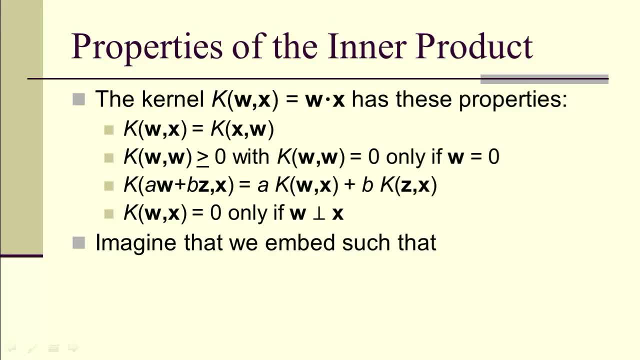 get around some of these conditions because we're embedding in a high-dimensional space. so what we can do is we can say: well, no training point is going to be mapped to the zero vector, so once we do our embedding, we're going to avoid the zero vector. so now we don't have to worry about the inner product of 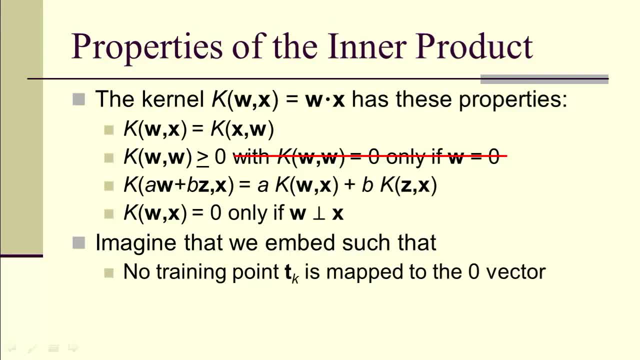 W with itself is 0 only if W is equal to 0. you, the embedding is nonlinear, so we're not going to try to preserve linear combinations, because we'll be looking at a nonlinear embedding that's being used in an inner product and we're just going to make sure that once we do the 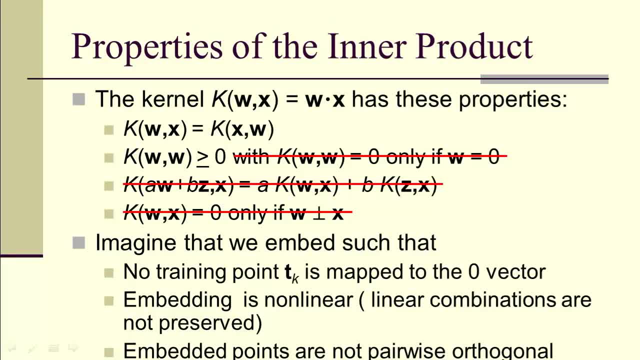 embedding. we don't get any orthogonality now. that means that we can do the embedding as long as we have symmetric and what's called positive definite or positive semi-definite. in other words, all we need is that the kernel function of w comma X is the same as the kernel of x comma W and that the kernel of w 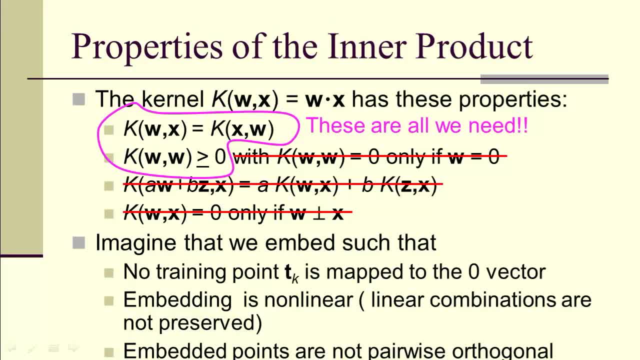 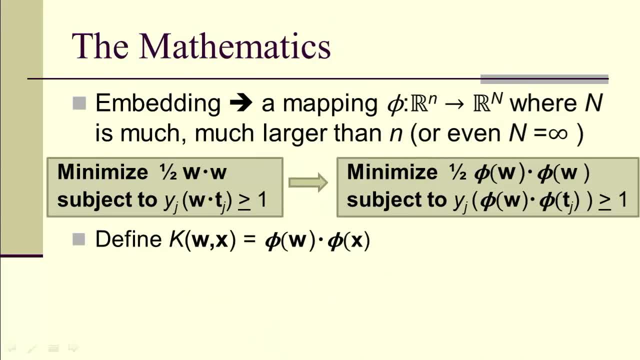 comma W is greater or equal to zero for all w's in this embedding space that we're eventually going to see. so now let's introduce our embedding. that's a mapping fee from our sub in to our sub capital in where the capital N is much, much larger than N. 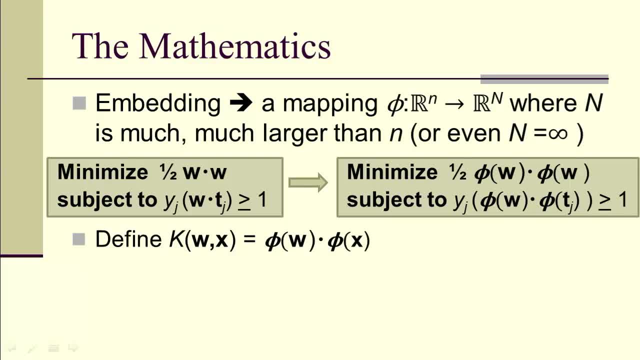 And in many instances we'll just let capital N be infinity, although we won't get into what it means to have an infinite dimensional vector space. So minimizing one-half W- dot W will be projected into the much, much larger space, into minimizing one-half phi of W- dot phi of W. 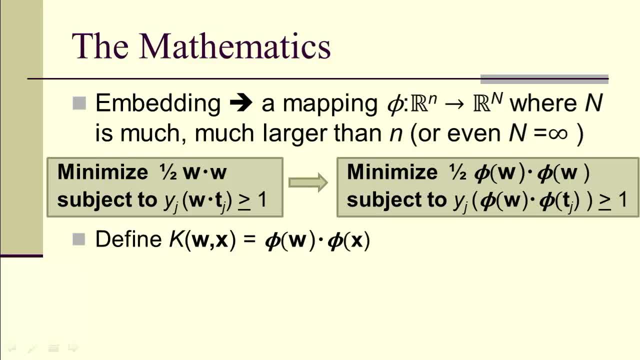 The boundary condition constraint likewise is going to be Y sub J phi of W, dot phi of T sub J, greater than or equal to 1.. So we're going to define our kernel to be the dot product of nonlinear images of W and X under this nonlinear embedding. 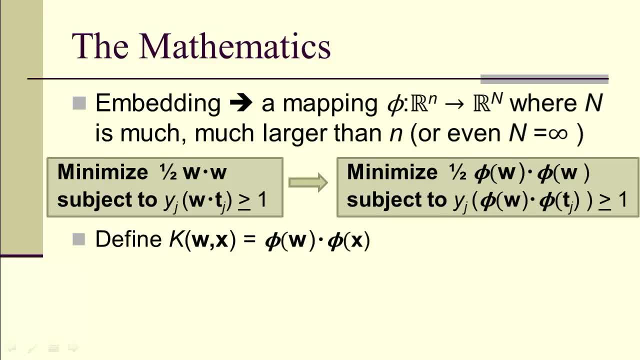 So K of W of X is equal to phi of W, dot phi of X, And that means we want to minimize over the scalars A sub J, subject to the boundary condition, And notice that our capital K here is in place of where the inner products were. 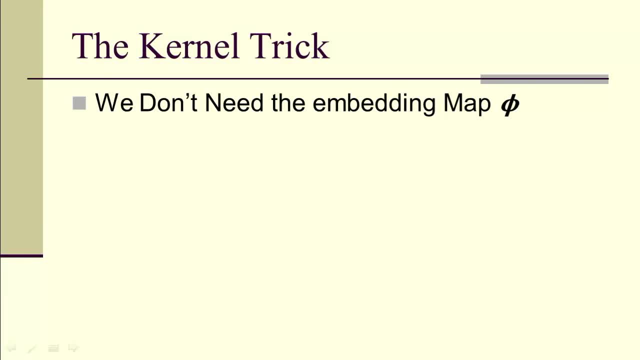 So the kernel trick is: if we do this, we don't need the mapping phi, We simply need a kernel. We simply need a kernel that has the same properties as phi of W, dot, phi of X for some extremely large value of capital N. 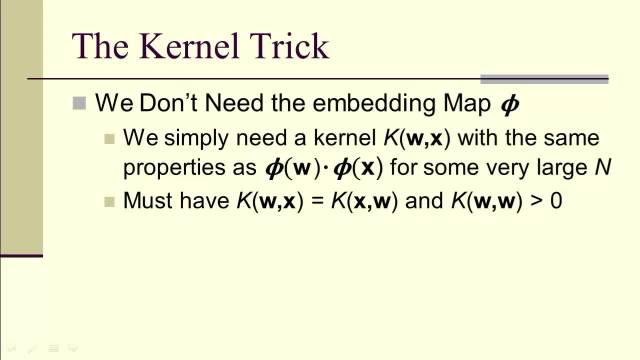 In other words, we have to have K of W of X equals K of X W and K of W comma W greater than or equal to 0.. So that brings up a thing called Mercer's condition, And I'm just mentioning this for completeness. 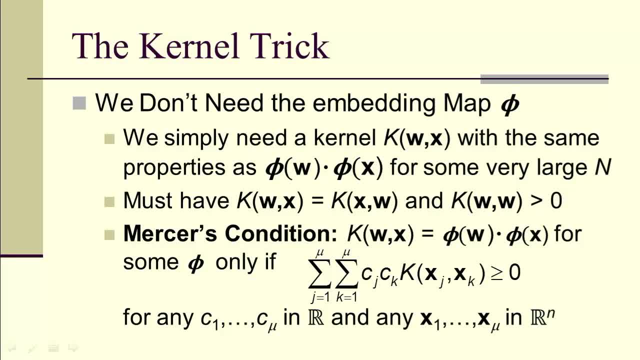 Mathematically it's a little beyond what we're trying to do in this introductory, But just so you'll know what to think about guaranteeing this K of W, dot W or K of W, comma W greater than 0,. the positive definiteness is a condition on the K, such that you get for any C1 to C mu in R and any X1 to X mu in R in. 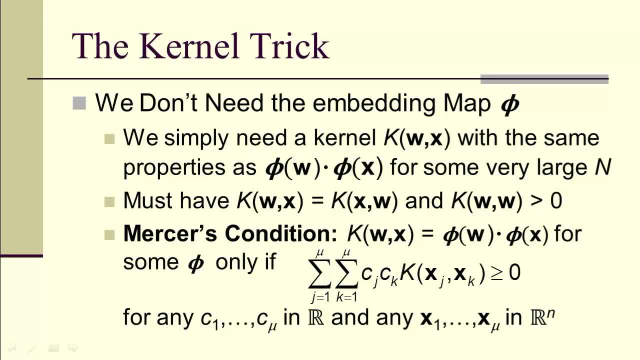 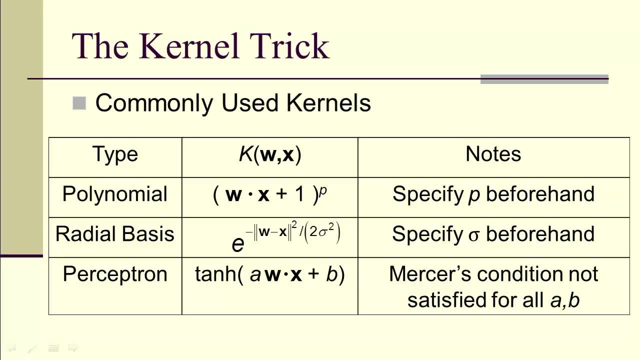 and this double summation is non-negative. So some commonly used kernels: Polynomial: You have to specify the degree of the polynomial beforehand. The radial basis: functions: You have to specify the value of sigma beforehand. Both of these have the nice property that they satisfy Mercer's condition. 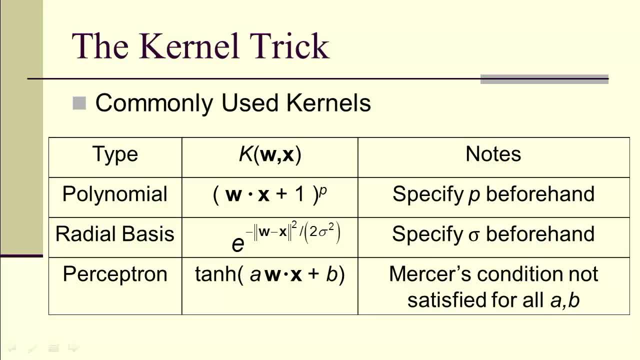 Now there's also one that's related to what's called a neural network- we'll see a little bit later- which is called the perceptron kernel, which is the hyperbolic tangent of A, of W, dot X plus B, And here, if you're going to use that, you'll have to check and make sure Mercer's condition is satisfied. 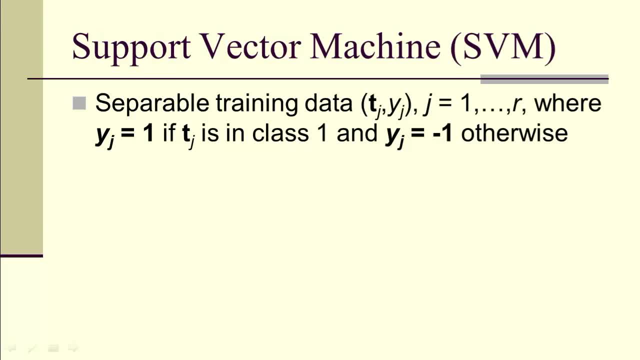 because it's not satisfied for all A and B. So now we have our support vector machine, Separable training data where Y sub J is 1 if T sub J is in class 1, and Y sub J is negative 1 otherwise. 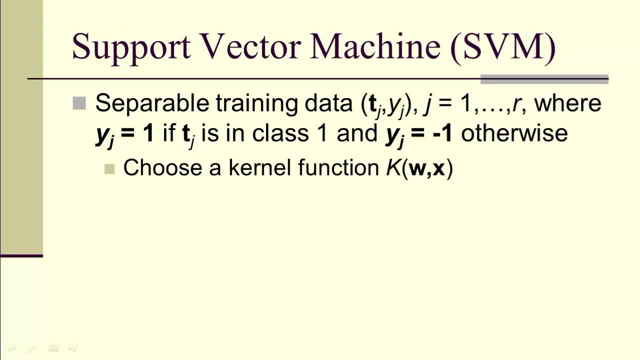 We choose a kernel function, It satisfies Mercer's condition and is symmetric. Then we want to find scalar coefficients- A1 to AR- and notice that this is only the size of the training data, not the size of the embedding space. So the embedding space can be enormously large, but still the number of independent variables for us is only equal to the size of the training data. So the embedding space can be enormously large, but still the number of independent variables for us is only equal to the size of the training data. So the embedding space can be enormously large, but still the number of independent variables for us is only equal to the size of the training data. 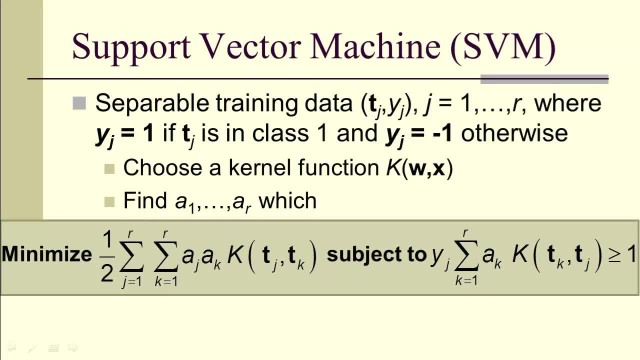 And so here's our problem: Minimize this: 1 half sum over J. sum over K is A sub J, A sub K times the kernel function of T sub J, T sub K. subject to our condition, Y sub J. sum K equals 1 to R, A sub K K of T sub K. comma. T sub J greater or equal to 1.. 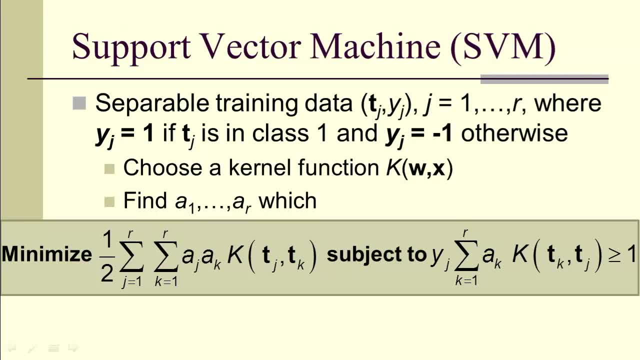 So the embedding doesn't appear explicitly. It's buried inside of this capital K, And that's the trick. And, once again, if you have coefficients which are not 0, then those are called support vectors. Now let me mention that this problem, while it's a very cool trick, it results in a problem which is called a quadratic program. 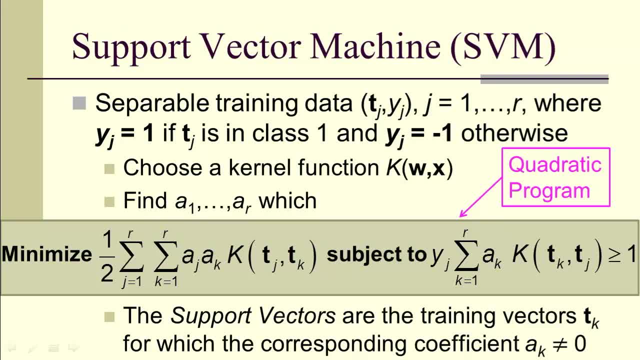 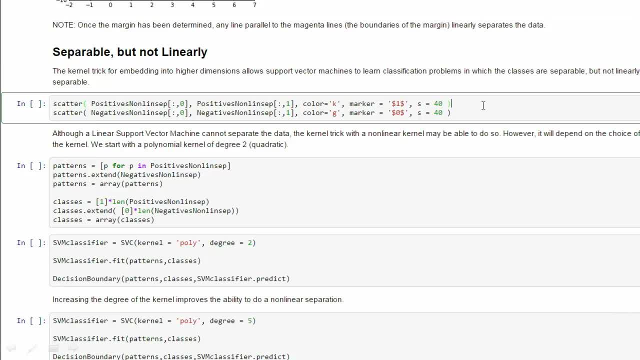 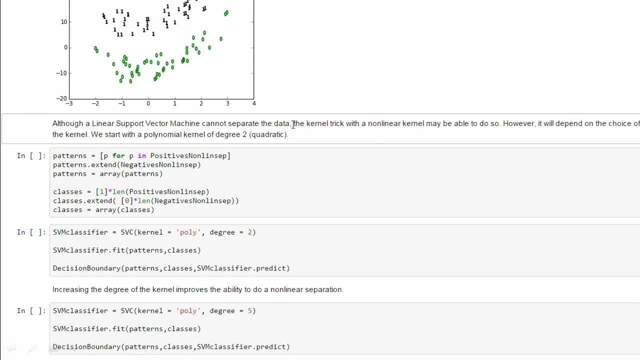 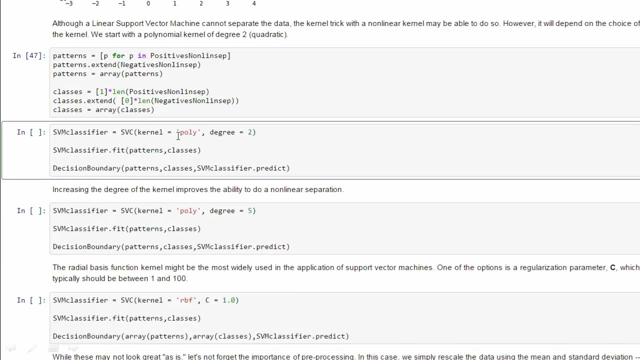 And this is a programming problem that's non-trivial but can be done. So let's look at an example. So when we loaded our notebook, notice we get some non-linear but separable data And you'll be playing with this when you play with the notebook later on. 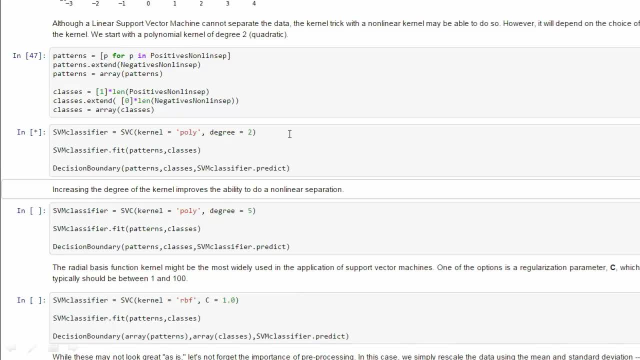 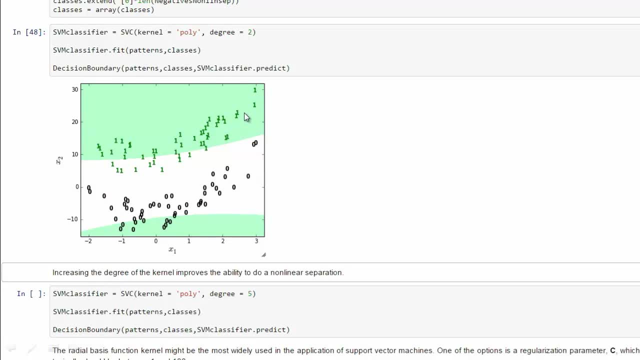 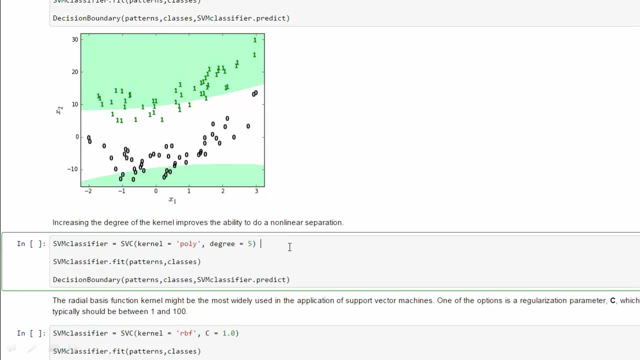 I'm going to start out with a polynomial kernel, just of degree 2, and it kind of looks like it's a quadratic And notice it doesn't do a very good job. So the choice of kernel is extremely important. So maybe a kernel 2 is too small. 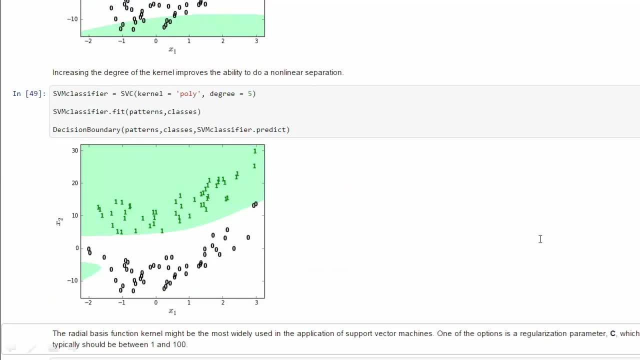 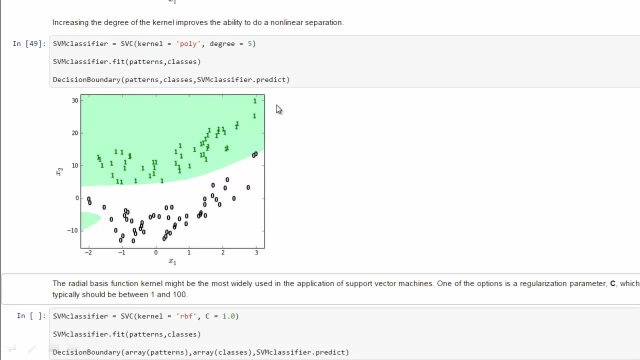 So we can see what happens with a degree of 5.. Well, that's a little better. At least it separates them, but it's probably not what we would think would be- quote- most natural. So let's use, instead of a polynomial, let's use a radial basis function. 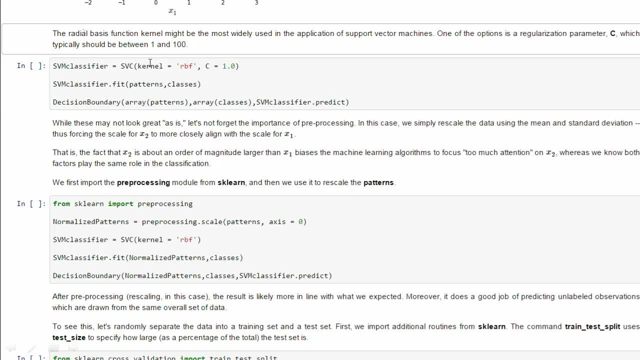 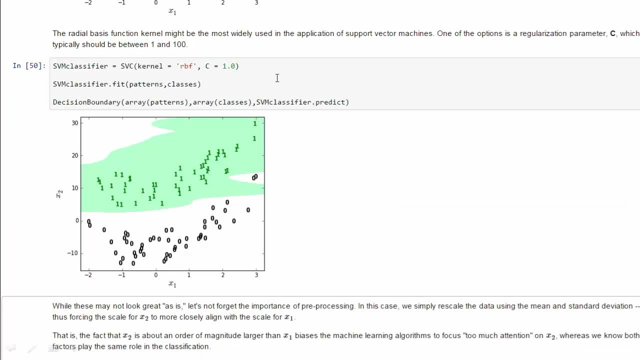 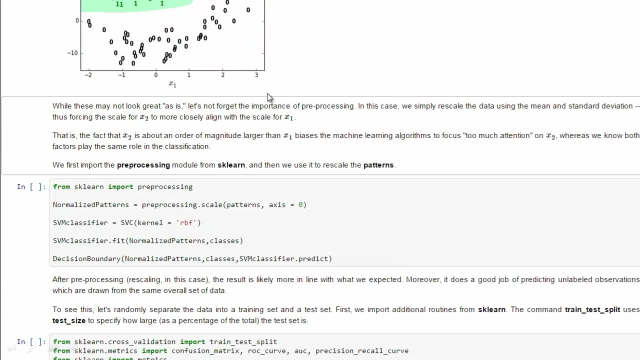 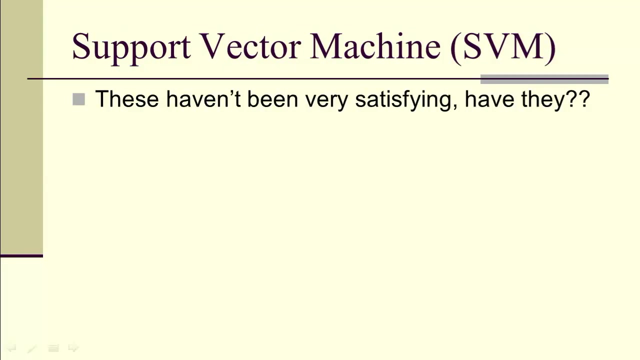 Now this is the one that's used very often. The embedding space is actually infinite dimensional And it has this regularization parameter And it actually does a pretty good job, but still not necessarily what we want. So we looked at three examples here with two polynomial kernels. 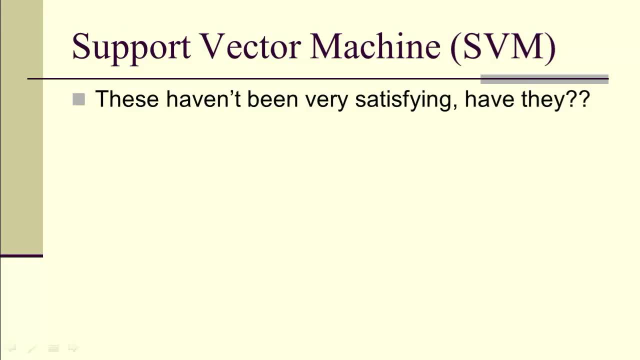 The first one didn't work at all. The second one was better, but still sort of a strange classifier, And the third one, the radial basis function, which I supposedly think is the greatest thing since sliced bread. it didn't work very well either. 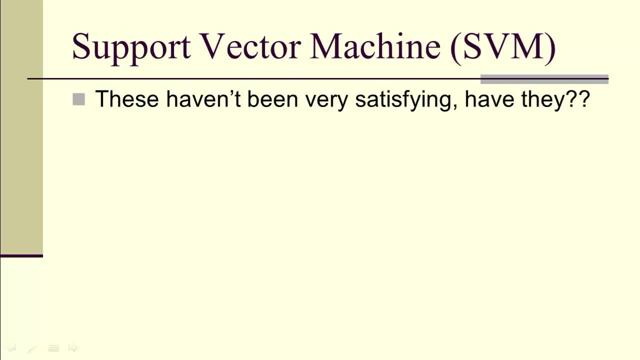 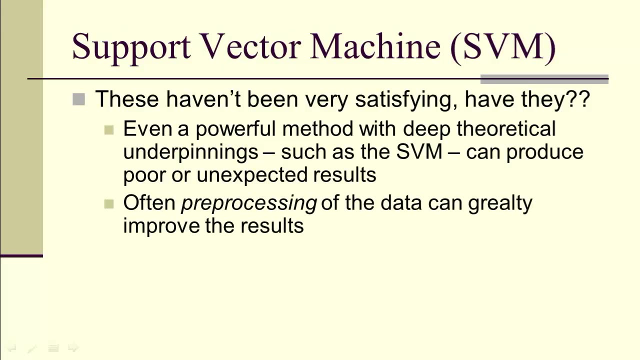 So why not? Well, one thing you have to keep in mind from way back in the earlier part of the course is that even extremely powerful methods can produce very poor or unexpected results, And very often pre-processing of the data can greatly improve the results. 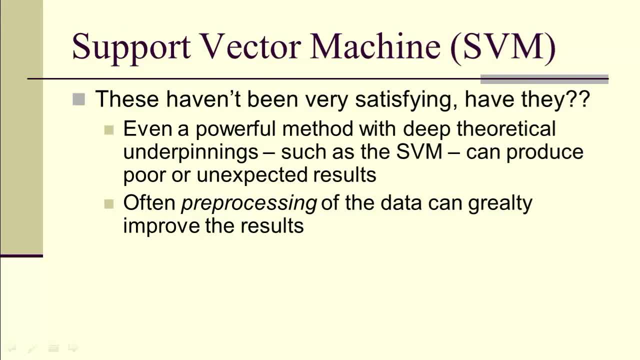 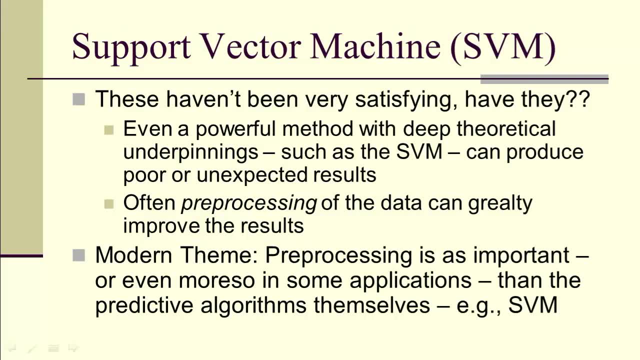 And very often, pre-processing of the data can greatly improve the results And very often, pre-processing of the data can greatly improve the results. This is a very important theme. Pre-processing is as important or even more so in some applications. 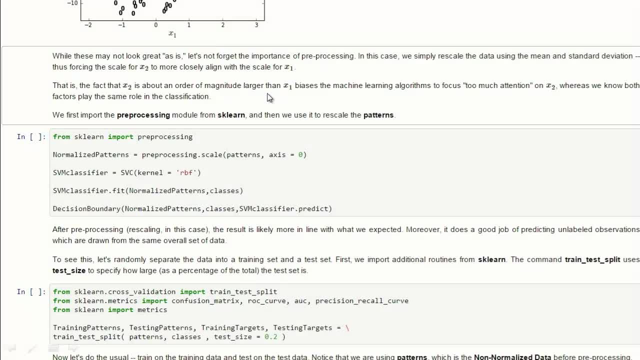 than the actual algorithms you use. So we're going to look at that, We're going to go back to the notebook And we're going to notice that the x1's go from negative 2 to 3 or so, but the x2's are an order of magnitude larger. 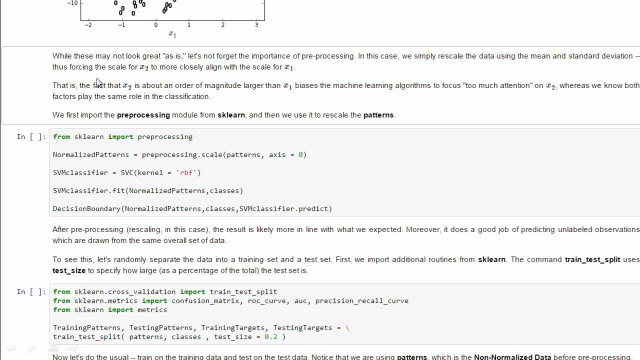 But the x2's are an order of magnitude larger. So we're going to preprocess by simply rescaling the x2 so that it more closely aligns with the x1. So we import preprocessing from our sklearn. here We normalize our patterns by rescaling them. 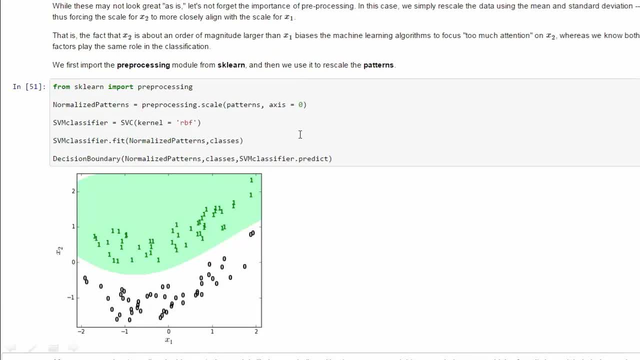 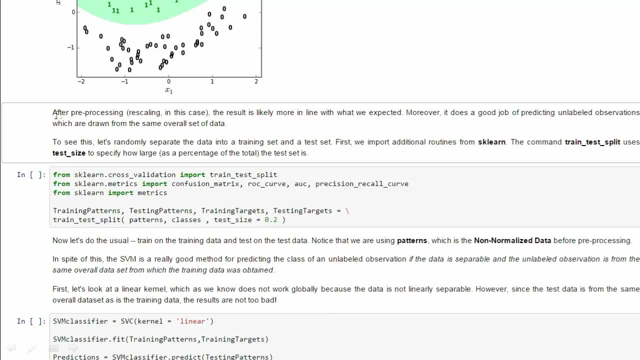 Now let's go back to our radio basis function. Oh, that's kind of nice. That's what we would have thought. Some sort of parabolic separator here. Some sort of parabolic separator here? okay, so the pre-processing really was a nice feature here. okay, now, once we start, 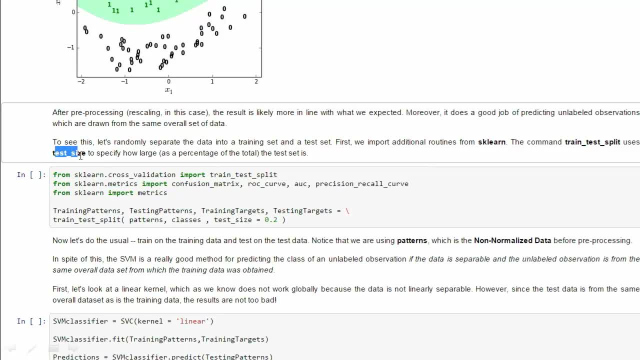 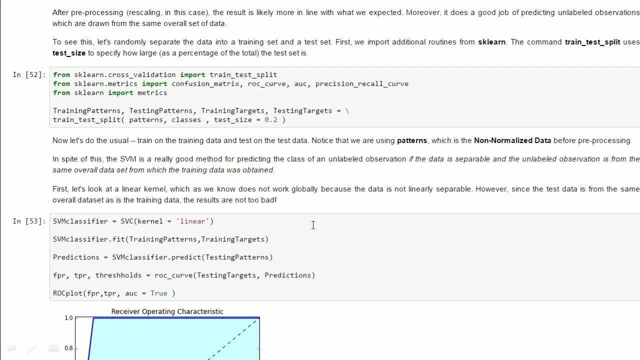 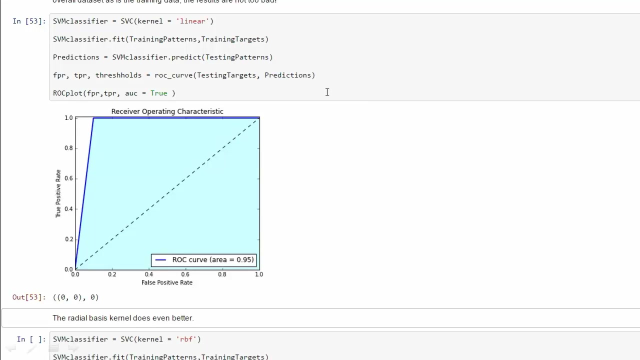 pre-processing. we also want to be sure that we're not simply getting results bomb the eyeball test, so we also want to start doing things like cross-validation. so now I'm going to look at this again using cross-validation, and our receiver operating characteristic on the testing data was point nine five that's. that's. 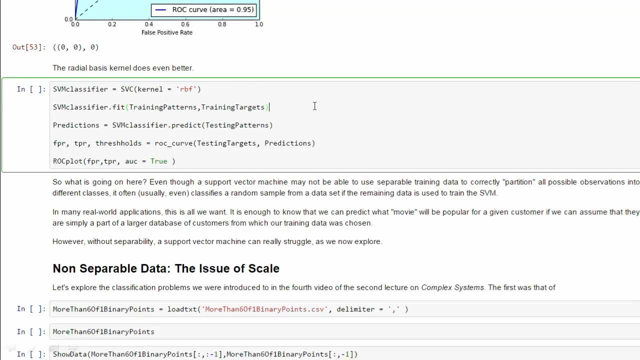 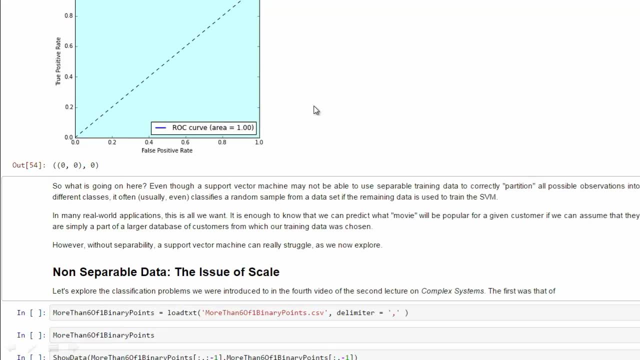 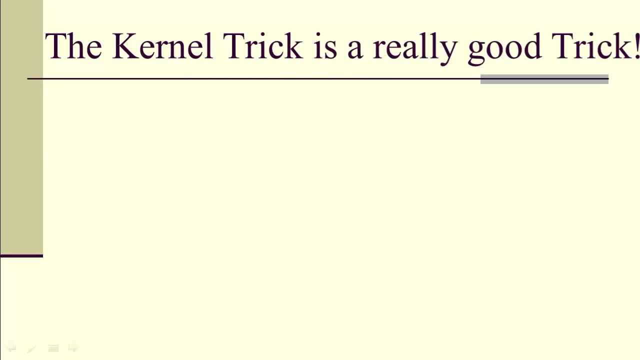 pretty good. radio basis functions actually perfect on the test data. so can't ever forget the importance of pre-processing. but of course, once we start pre-processing we really need some kind of a cross validation, because pre-processing is always a source of bias or can be. so the kernel trick: it's a really good trick.